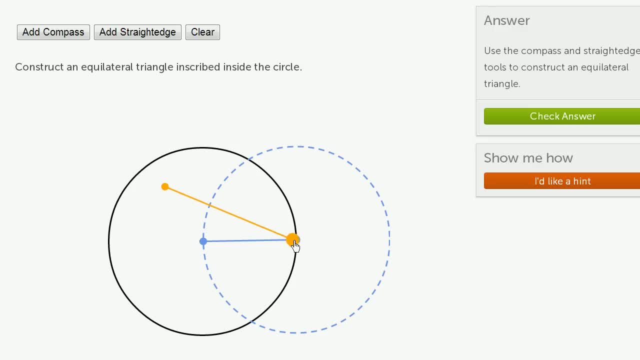 And that's either of their radii, because they have the same length. Now let's center this at our new circle and take it out here. Now, this is equal to the radius of the new circle, which is the radius same as the radius of the old circle. 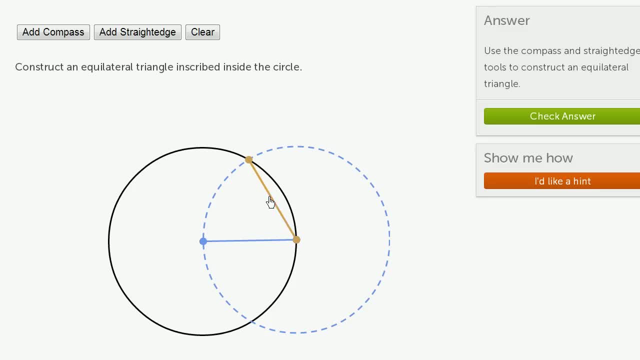 It's going to be the same as this length here, So these two segments have the same length. Now, If I were to connect that point to that point, this is a radius of our original circle, And so it's going to have the same length as these two. 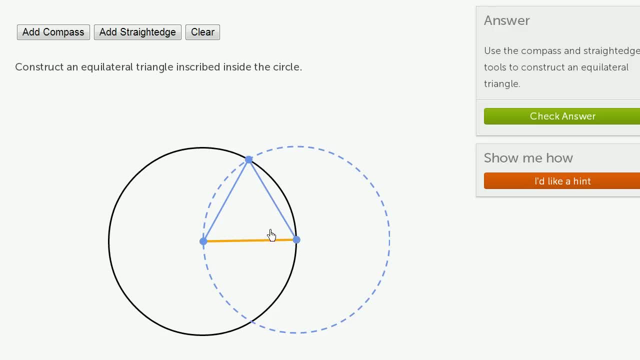 So this, right over here, I have constructed an equilateral triangle. Now why is this at all useful? Well, we know that the angles in an equilateral triangle are 60 degrees. So we know that this angle right over here is 60 degrees. 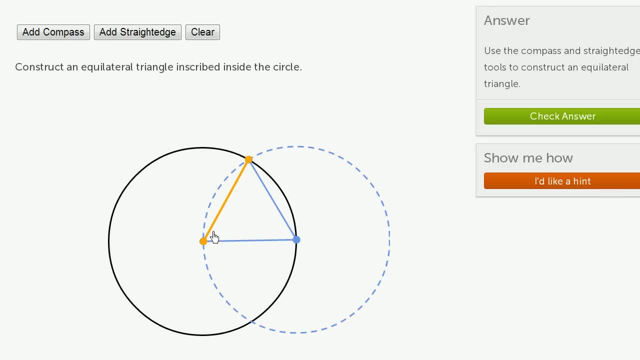 Now, why is that? Why is this? Why is this being 60 degrees interesting? Well, imagine if we constructed another triangle out here, just symmetrically but kind of flipped down, just like this. Well, the same argument, this angle, right over here. 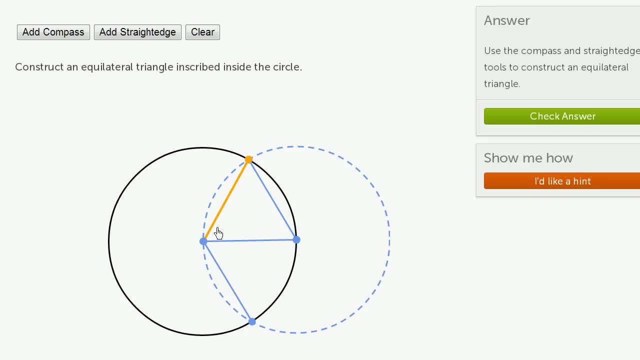 between these two edges. this is also going to be 60 degrees. So this entire interior angle, if we add those two up, are going to be 120 degrees. Now why is that interesting? Well, if this interior angle is 120 degrees, 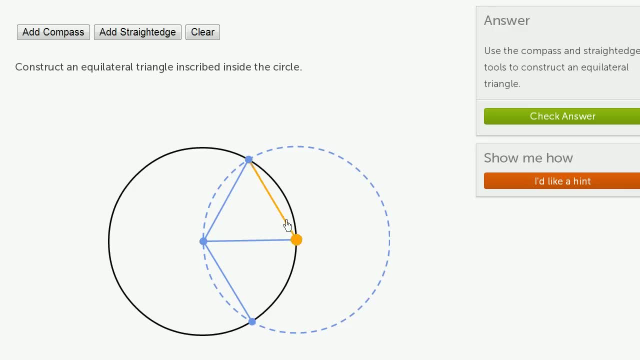 then that means that this arc right over here is 120 degrees, or it's a third of the way around the triangle. This right over here is a third of the way around the triangle. Since that's a third of the way around the triangle, 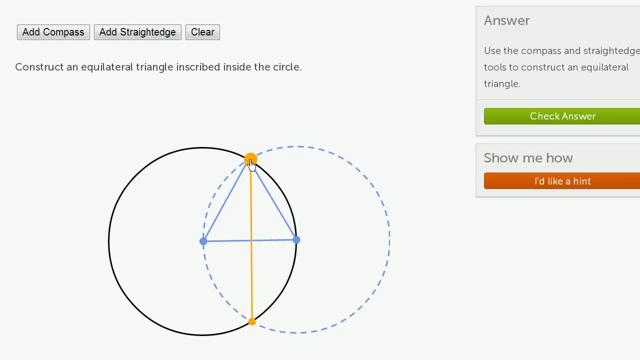 if I were to connect these two dots, that is going to be. this right over here is going to be a side of our equilateral triangle. It's this right over here. It's secant, It's to an arc that is 1 third of the entire circle. 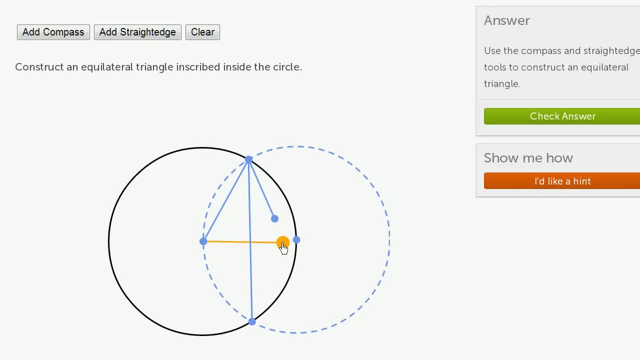 And now I can keep doing this: Let's move, Let's move, I'll reuse these. Let's move our circle around. And so now I'm going to move my circle along the circle. And what I want again, I just want.